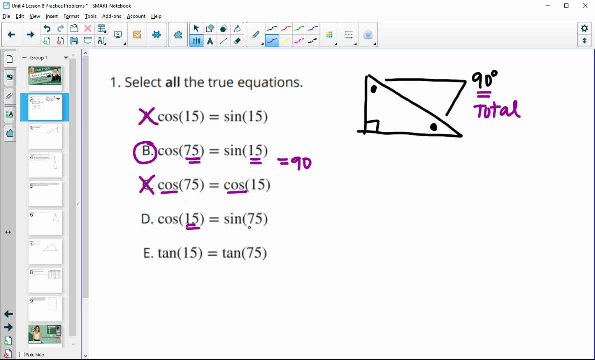 Cosine of 15 and sine of 75, that's going to be good, because 15 plus 75 equals 90. And then in part E it's tangent, So that one's not going to work. has to be a sine and a cosine. 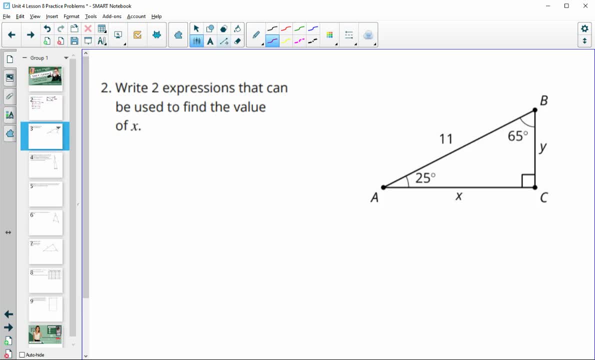 So, number two: write an expression that can be used to find the value of X, or write two expressions, sorry So, any two expressions. Now there's going to be a ton of them that will work for this. You've learned a lot of ways to solve for a missing side. 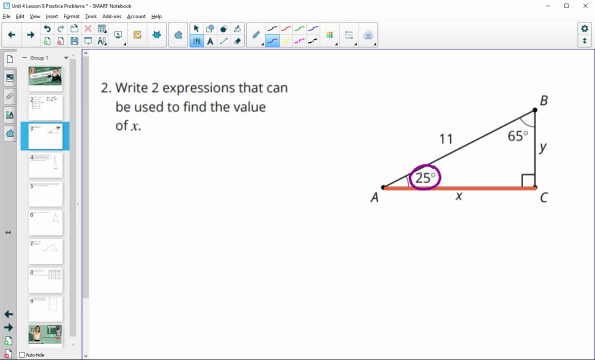 So in here you could do if you wanted to use the 25 degree angle as your anchor point, then X is going to be the adjacent side And then you've got the 11. So you'd have adjacent and hypotenuse if we're looking at the 25 degree angle. 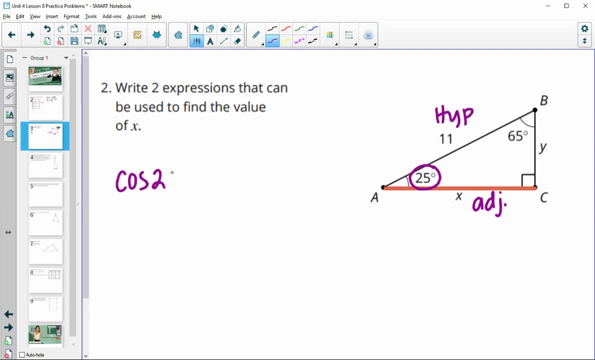 And our cosine function puts together the adjacent and the hypotenuse. So it's going to be: cosine of 25 equals the adjacent X divided by the hypotenuse 11.. Then if you wanted to use the 65 degree angle, now, the side with the X is the opposite side. 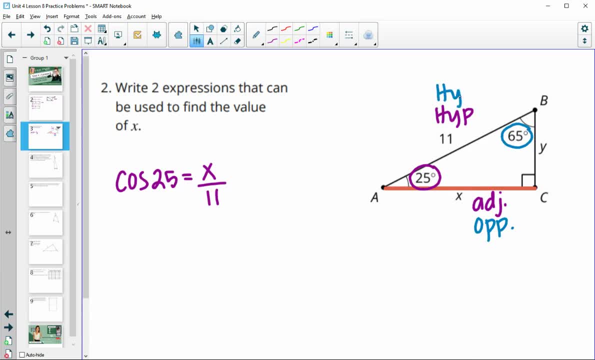 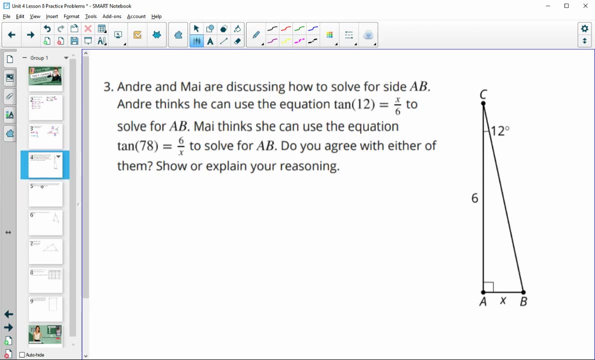 And then the 11 stays the hypotenuse. So opposite, and hypotenuse is our sine function. So we would do: sine of 65 equals X over 11 if we wanted to do it that way. Number three: Andre and Maya are discussing how to solve for side AB. 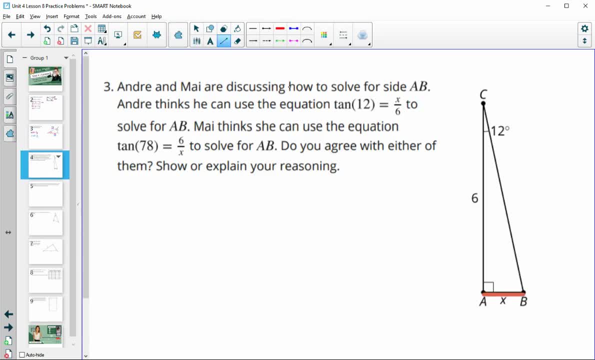 So AB is the one labeled X on here, And Andre thinks that you can use the equation of tangent of 12 equals x over 6 to solve for AB, and Mai thinks that you can use the equation tangent of 78 equals 6 over x. Do you agree with either of them? Show or explain your. 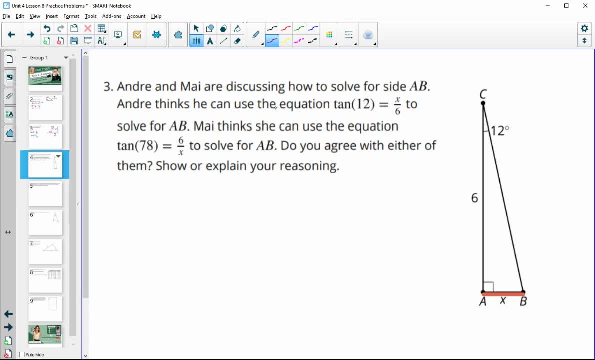 reasoning. So if we take a look first at Andres, he's looking at the 12-degree angle. okay, So here's the 12-degree angle. The x would be opposite of that angle, since it's directly across the triangle, and then the 6 is the adjacent side because BC is the hypotenuse, So opposite, and 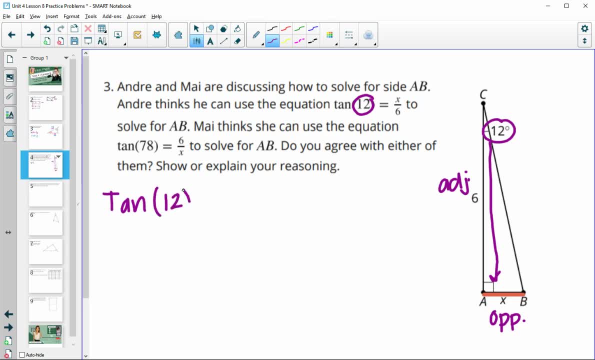 adjacent is a tan function. so we would do: tangent of 12 equals the opposite x over the adjacent 6, and that is the equation that Andres said. So Andres is going to be good. Then we can look at Mai's and she thinks the equation tan 78 equals 6 over x. So 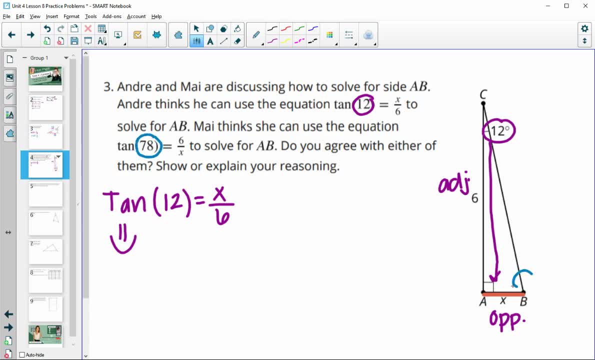 they're going to be good, So they're going to be good, So they're going to be good. So this 78-degree angle is coming from angle B, since 90 minus 12 equals 78 for that angle. So in this case, when we're looking at angle B now, directly across from angle B, is the 6.. 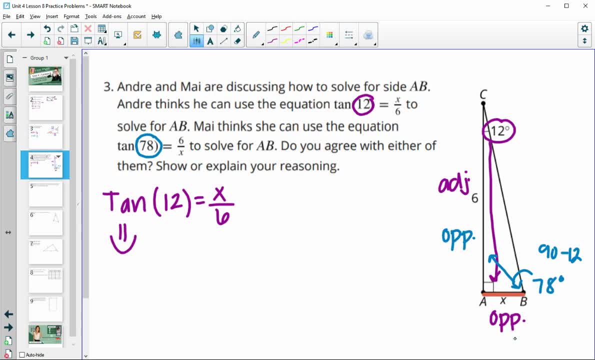 So this side is opposite of angle B and the x is adjacent to angle B. So if we do the tangent of 78, the opposite side goes on top, which is the 6, and the adjacent side on the bottom, which is the x, and that is the equation. 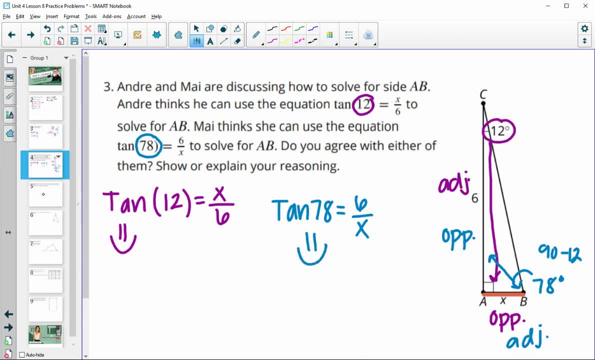 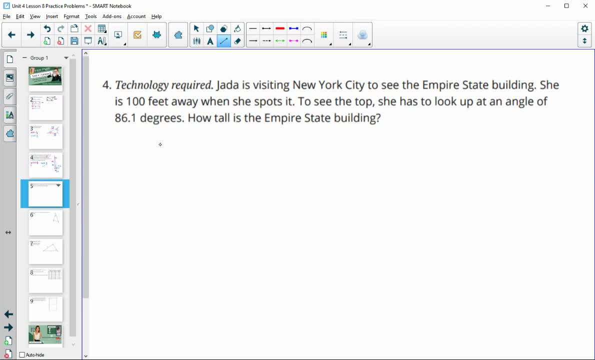 that Mai set up, So that equation is going to be good as well. Number four: Jada is visiting New York to see the Empire State Building. She's 100 feet away from the spot where she sees it and when she looks to the top of the building. 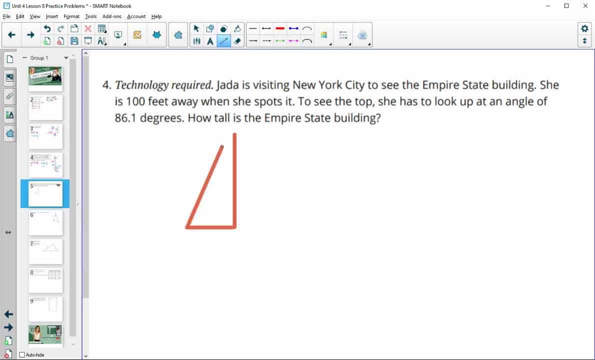 she needs to look up at an 86.1 degree. So how tall is the Empire State Building? So we know this length right here is 100 feet, and we also know this angle: here is 86.1 degrees, And then we're looking for this height. 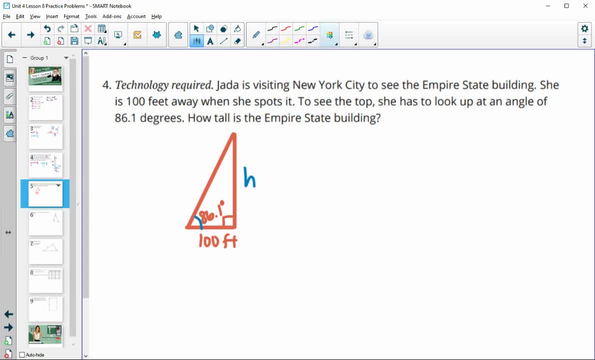 So this is the angle that we're given. So let's label the sides. I'm just going to change that to orange. So directly across from this angle is the opposite side, So the height is the opposite, And right next to the 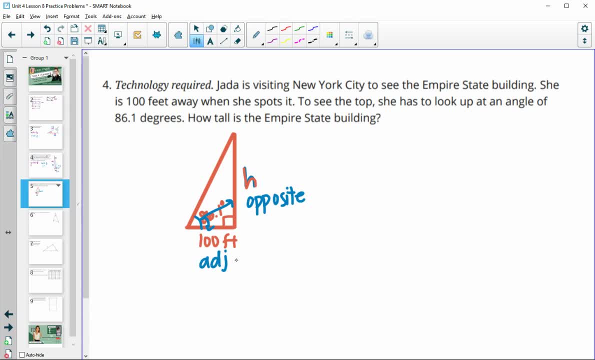 angle is the adjacent, So the 100 is the adjacent. So the function that puts together the opposite side and the adjacent side is the tangent function. So we'll do: tangent of the angle equals the opposite side divided by the adjacent side, And in this case our angle is 86.1 degrees. 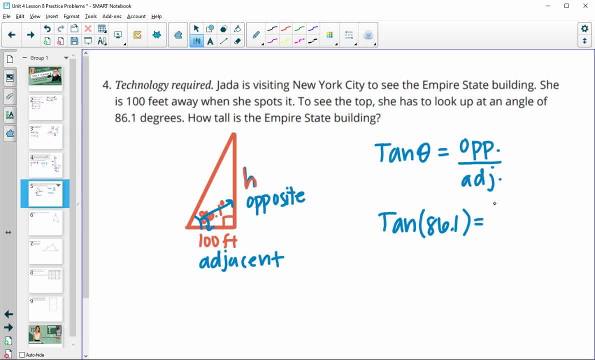 That's going to equal the opposite side, h over 100.. And so then, if we type in tangent of 86 into our calculator, this is 14.67 feet, And then we can just cross, multiply. So multiply this 100 up. 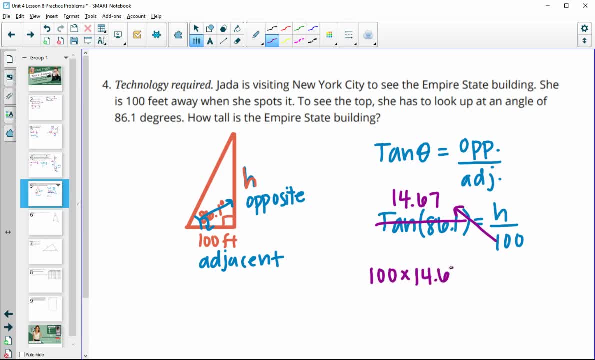 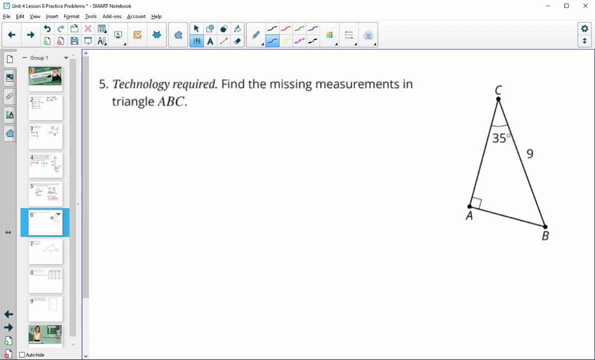 So we'll do 100 times 14.67. To get our height. So the height is 1,467 feet. Number five: find the missing measurements in this triangle. So we'll go ahead and look for side AB, We'll also look for side AC And then we will also look for angle B. 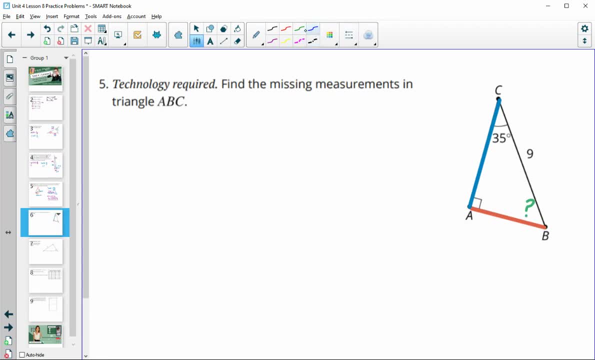 So I like to use the information that's given to me. So I'm going to use this 35-degree angle And I'm going to solve for the orange side first. So directly across from the angle, is the opposite side. So this side, AB, is the opposite side, And then the side that was given. 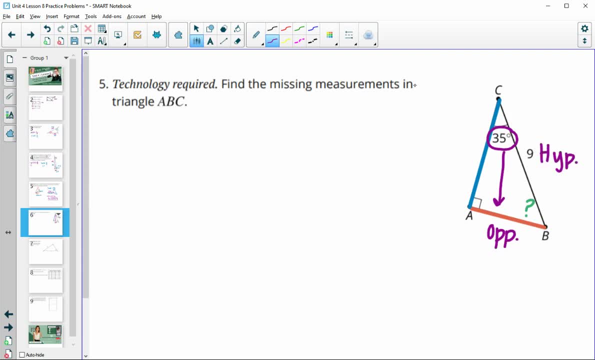 to us this nine is the hypotenuse. So the function that connects the opposite and the hypotenuse is the side AB, And then the side that was given to us this nine is the hypotenuse, And then the side that was given to us this nine is the sine function. So sine of our angle is: 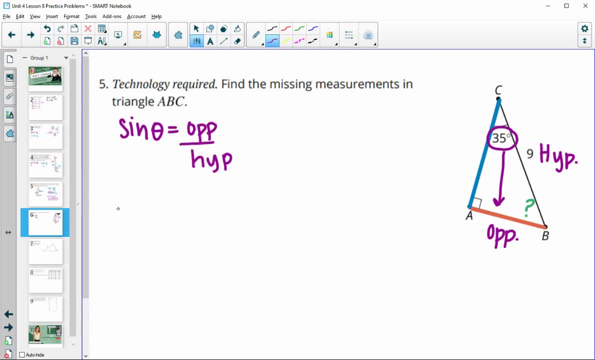 going to equal the opposite over the hypotenuse. So sine of 35 is going to equal our opposite side, AB divided by our hypotenuse of nine, And the sine of 35 is equal to 0.5736.. If we type that, 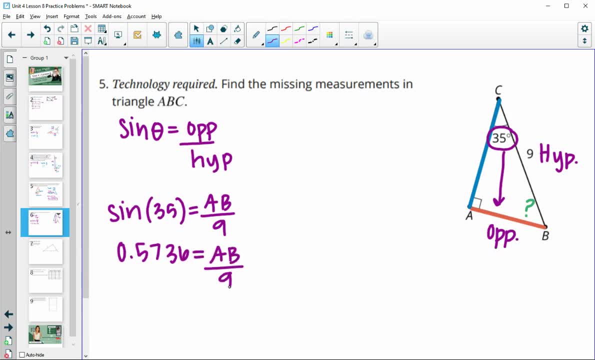 into our calculator. Then we just need to multiply this nine up, So we'll do nine times the 0.5736.. And that will give us about 5.16 for side AB. Then you have a couple of options to find the blue. 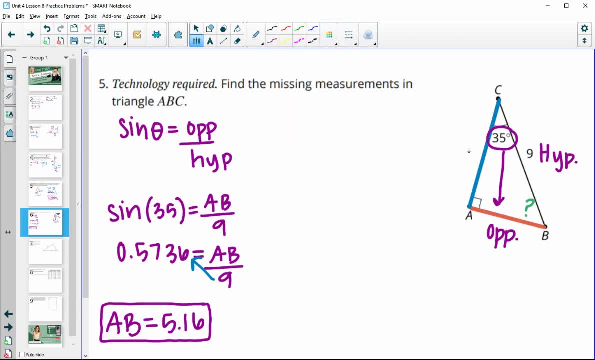 side, You could set up a cosine function, since that's the adjacent, Or you could do the Pythagorean theorem. So I'm just going to set up the cosine function actually. So cosine of 35 is equal to the adjacent side, which is AC, over the hypotenuse, which is nine. 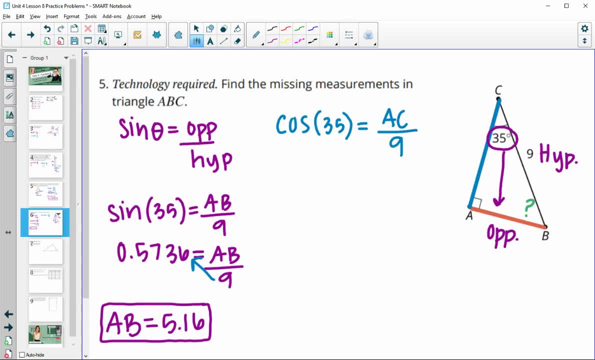 And so type in the cosine of 35 into your calculator and you'll get 0.8192 is equal to 0.8192.. AC over 9.. So then we can cross, multiply that 9 up and we'll do 9 times 0.8192. 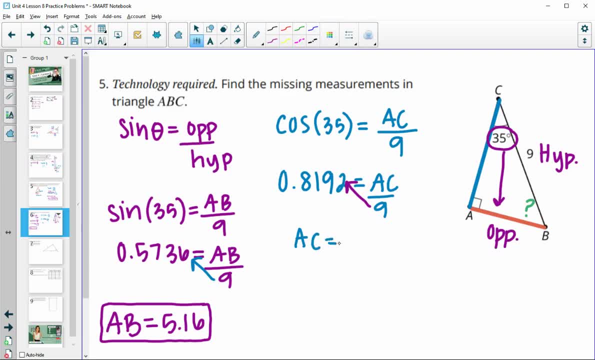 and we get that side AC is equal to about 7.37.. Then the last thing we need to solve for is that missing angle. So we know that angle B and C in a right triangle total 90. So angle B is going to equal 90 minus that 35. So angle B is going to be. 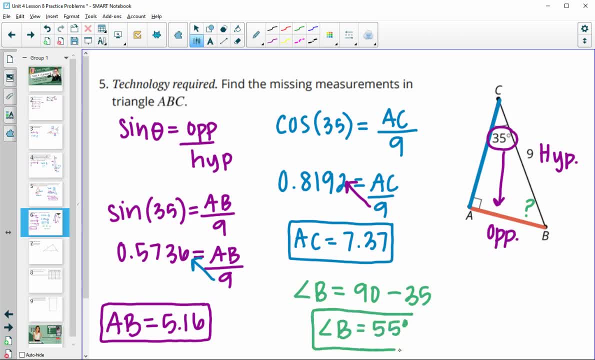 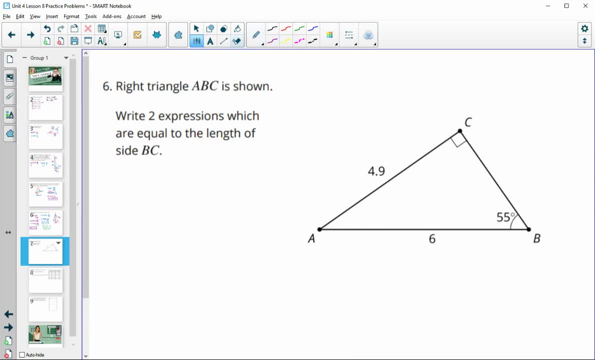 55 degrees. Number six: write two expressions to find the length of BC. And so we've got quite a few things we can do here. But if we use this 55 right away, then I could label the 4.9 the opposite and the sixth the hypotenuse. So you could set up with that. 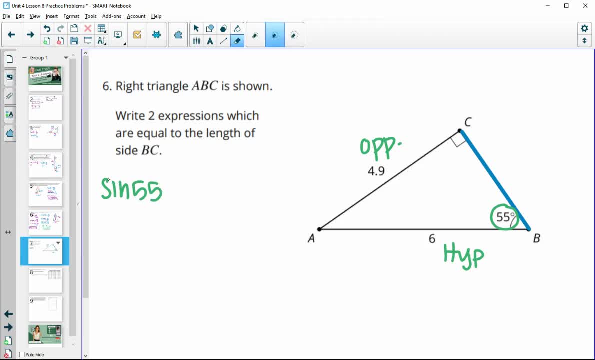 55 degree angle. a well, we don't want to do a sine function actually, because that's the opposite of the hypotenuse, But we could do a cosine function. So if we do cosine of 55, cosine is the adjacent which is side BC over the hypotenuse. 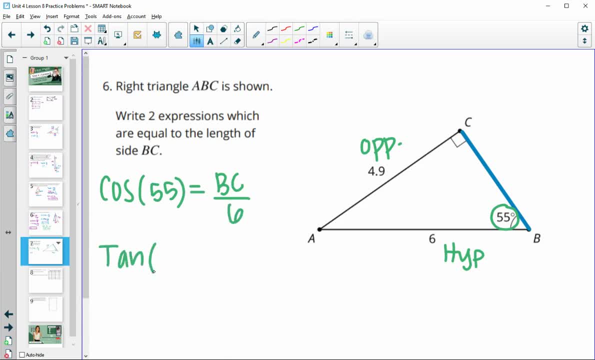 which is the opposite of the hypotenuse. So if we do that, then we could set up with that 55 degree angle, Which was six. We could also do a tangent function. So tangent of 55 equals the opposite, which is 4.9, over the adjacent, which is BC. So that would be two equations there. So you'd. 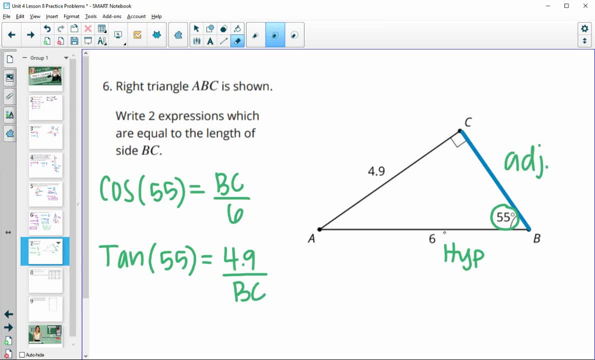 certainly be done with the problem. if you wanted to use those, You could also go ahead and look at this angle. So we could do 90 minus 55. Which would give us 35 degrees here, in which case the six would stay the hypotenuse, But now BC would be the opposite and 4.9 would be the adjacent. So we could say the sine of 35 is equal to the opposite BC over the hypotenuse of six And you could do a tangent function of 35.. Which would give us 35 degrees here, in which case the sine of 35 is equal to the opposite BC over the hypotenuse of six, And you could do a tangent function of 35.. Which would give us 35 degrees here, in which case the sine of 35 is equal to the opposite BC over the hypotenuse of six, And you could do a tangent function of 35.. 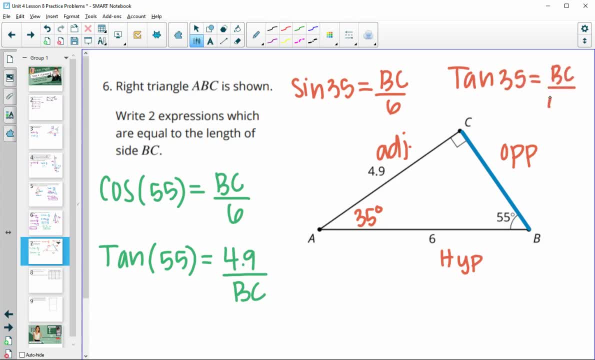 So then in this one we also have the two sides given to us, So we could also look into doing a Pythagorean theorem, And so the expression here would be that C squared equals A squared plus B squared. But if we solved it for BC, we know we would get the square root of the hypotenuse squared. 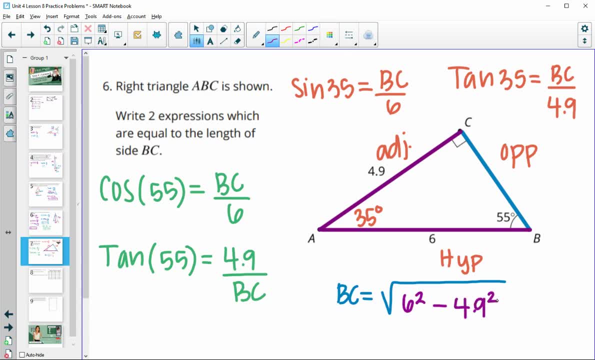 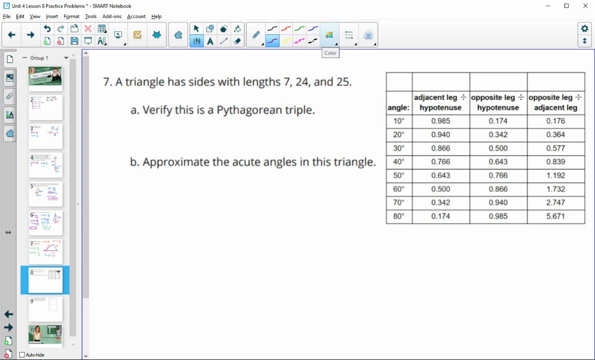 squared minus the leg squared, So you could do square root of 6 squared minus 4.9 squared for an equation as well. All right, in number 7, we want to verify that a 7,, 24, 25 triangle is a Pythagorean triple. So remember, we'll plug this into Pythagorean theorem. So 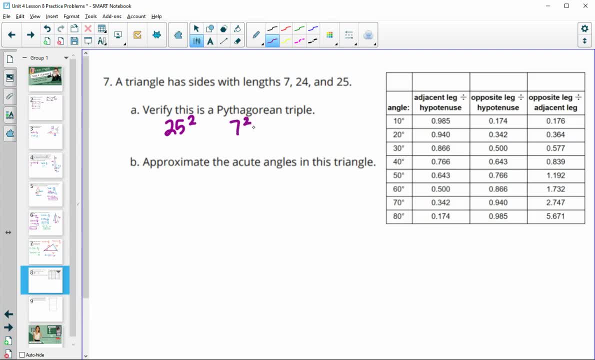 taking a look at 25 squared and then at 7 squared plus 24 squared. So 25 squared is 625.. 7 squared is 49 and 24 squared is 576.. When we add 49 and 576, we get 625.. So then, that verifies. 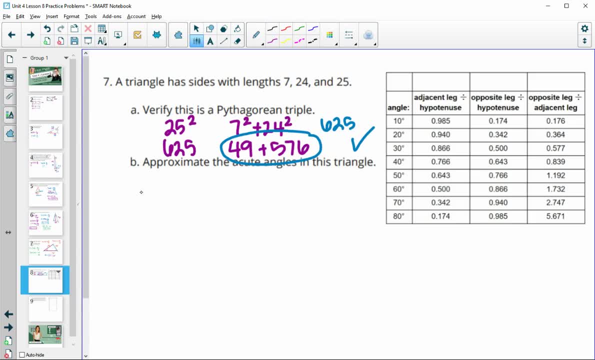 that it's a Pythagorean triple. Then we want to actually approximate the angles in this right triangle, So you can just draw a sketch if you need to. So this would be 7,, 24, and then 25.. And then I'm just going to label an angle, just so that I can kind of see what I'm doing. 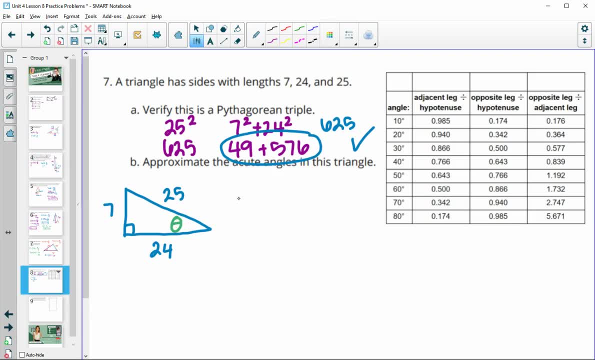 So in this, if I'm looking at finding this angle here and I do, 7 divided by 24.. So 7 divided by 24 as a decimal gives us 0.2917.. And the 7 is our opposite side. 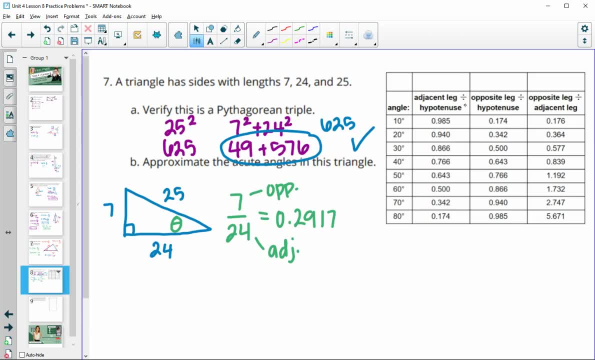 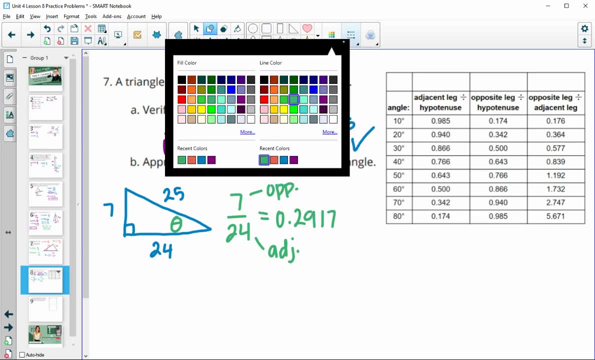 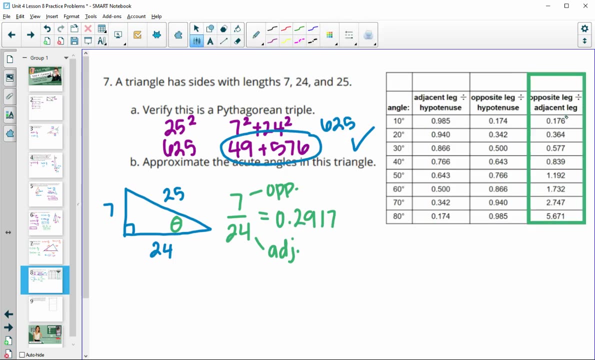 And the 24 is our adjacent side. So we would be looking in the opposite, over adjacent column, And then we'd be looking for the decimal of 0.29.. So we can see that that's somewhere between these. So about like 15 or 16 degrees. So if we just said 16 degrees here, 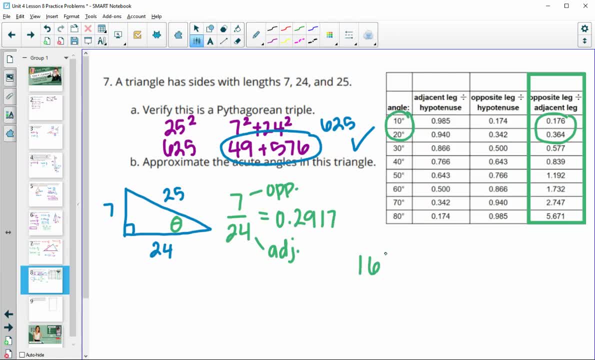 then we have a coupe and then we have a triple. So we would be looking at 7 squared plus 15, that from 90.. So 90 minus 16 would give us 74 degrees for the other angle. So then those would be some approximations there, All right. And then number eight says Priya is playing handball and 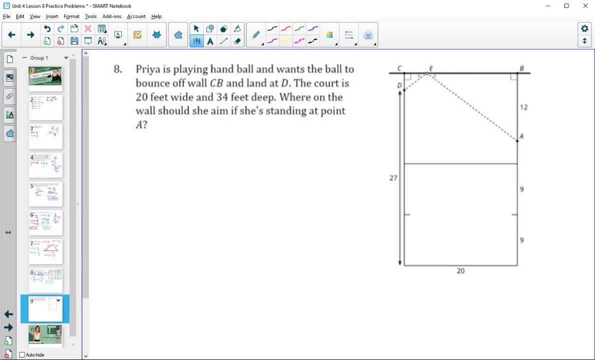 wants the ball to bounce off wall CB at point E. The court is 20 feet wide and then 34 feet deep, So this is 34.. Where should she hit the ball? Okay, So where should she hit the ball if she's? 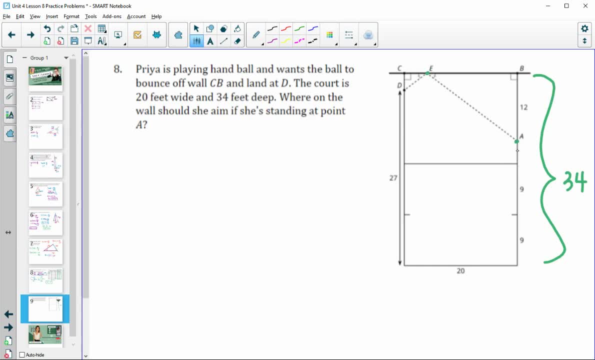 standing at point A. So first thing we need to do is figure out how big this is. So we know this length here is 12.. and then we want to compare it to the comparable side or the corresponding side over here. So we know that the whole length is 34.. So we're going to do 34 minus 27 and we'll get that this. 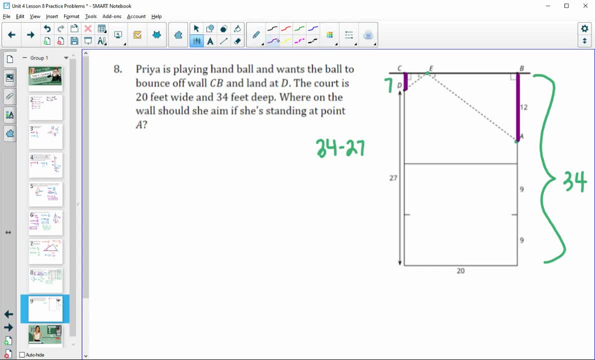 length right here is 7.. So then we're going to be comparing 12 to 7, and then we also want to compare these other lengths over here, So this one and this one, and we know the total is 20 for those, So the one that we're trying to see. okay, so where should she aim if she's standing at 0.8??